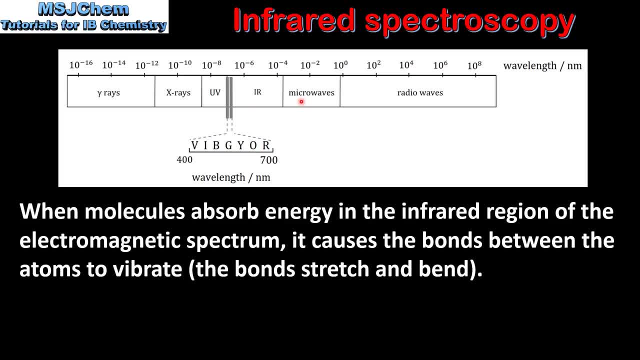 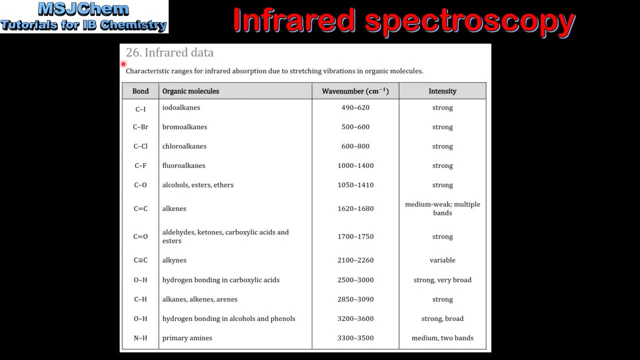 and we can find infrared radiation between microwaves and visible light. The frequency of infrared radiation that is absorbed is measured as the number of waves per centimeter. This is known as the wave number. In table 26 of the data booklet you'll find all the information that you need to solve problems for infrared spectroscopy. 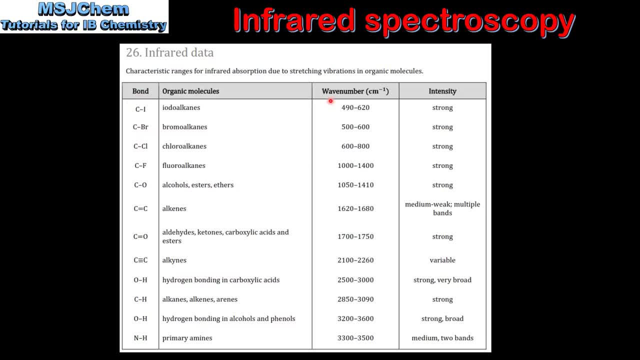 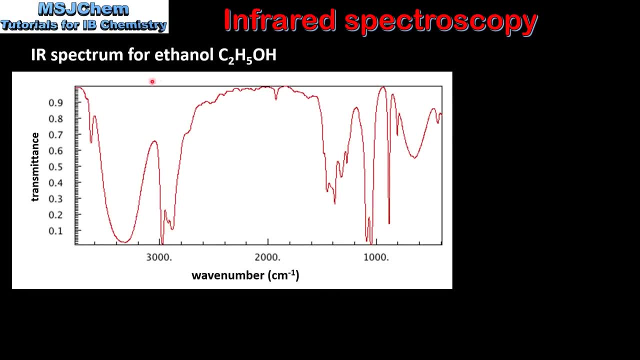 We have the type of bond, the organic molecule, the wave number and the intensity. So here we have an example of an infrared spectrum, this one being for ethanol. On the y-axis, we have transmittance. On the x-axis we have wave number. 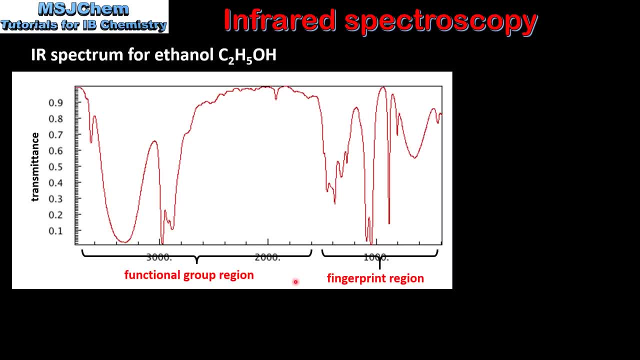 The infrared spectrum can be divided into two regions. On the right we have the fingerprint region. On the left we have the functional group region. The fingerprint region is the region of an infrared spectrum in the range of about 500 to 1500 centimeters to the negative one. 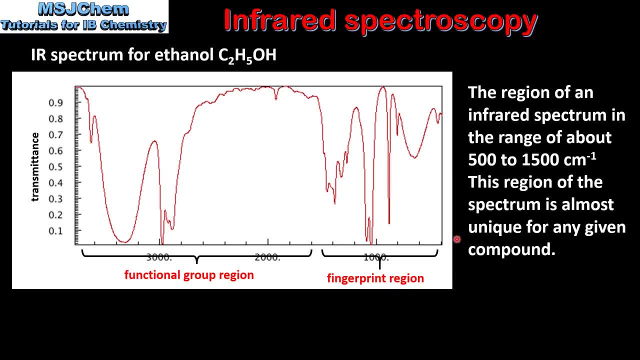 This region of the spectrum is almost unique for any given compound. The fingerprint region can be used to identify an unknown compound by comparing with the infrared spectra of known compounds. The functional group region gives information about the type of bonds that are present within the molecule. 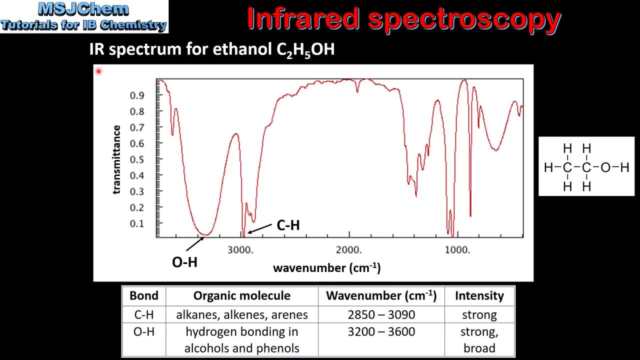 Next, we'll use an infrared spectrum to identify the bonds in a molecule. So by looking at the wave number of the peaks and comparing to the data in the table, we can determine which bonds are present in the molecule. So this peak occurs at a wave number of approximately 2,000 miles per second. 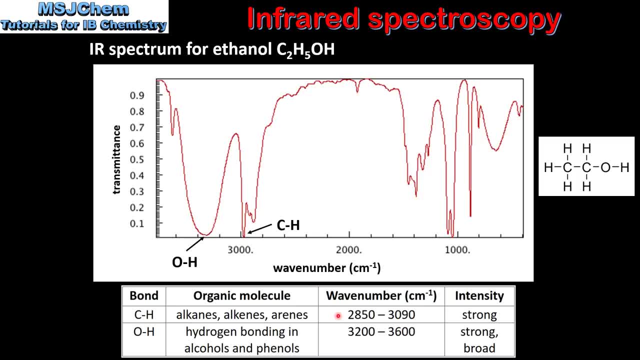 This peak occurs at a wave number of approximately 3,300 centimeters to the negative one. By looking in the table, we can see that this wave number corresponds to a carbon to hydrogen bond. The next peak occurs at a wave number of approximately 3,300 centimeters to the negative one. 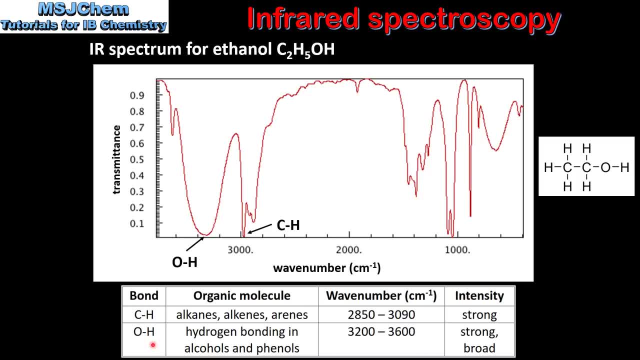 So once again we look in the table and this wave number corresponds to an OH bond in alcohols and phenols. So from this infrared spectrum we've determined there's an OH bond and a CH bond in the molecule. And if we look at the structural formula for ethanol,